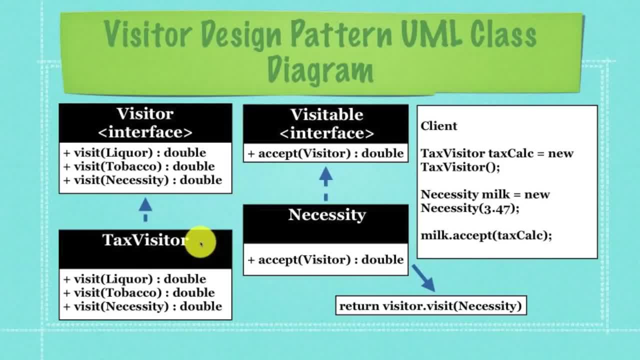 and our job is to implement taxes, However, implement them in a way so that different types of products- being either liquor, tobacco or necessity items- are taxed in completely different ways. And then what we're going to do is create the visitable interface, and it is going to have a method that every class that implements, it being either 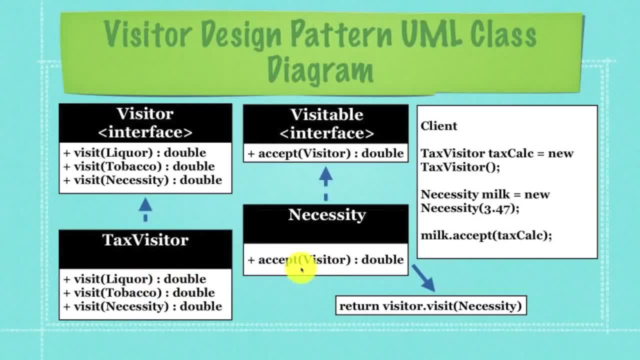 necessity. tobacco or liquor is going to have that accept method inside of it. So let's look over here at what the client's going to do. to further explain what's going on over here. First, we're going to create tax visitor, which you can see in the lower left hand corner of your screen. 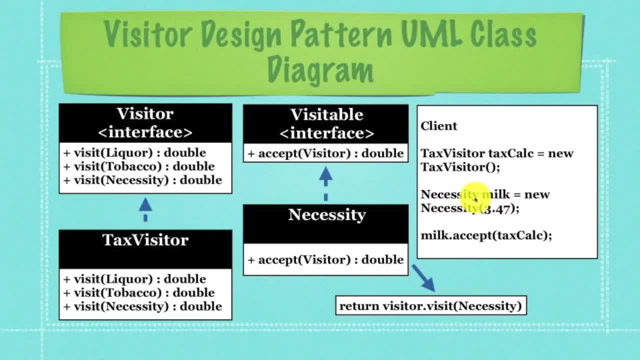 and then we're going to define one of our class objects. So we're going to define milk as a necessity and we're going to say that it has a price of three dollars and five cents. So we're going to come over to the readiness window and I'm going to say the price you want to see will be. 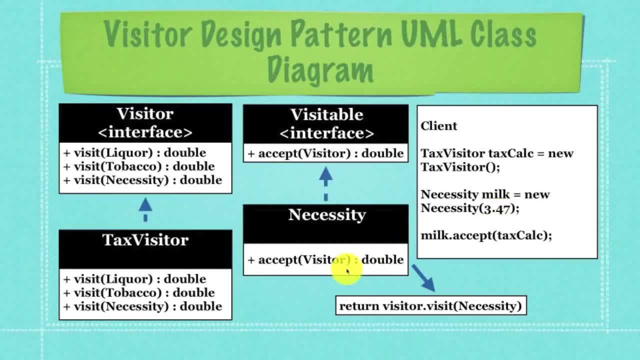 three dollars and forty-seven cents a gallon. What, then, is going to happen? is this three dollars and forty-seven cents is going to come over here, and how we get this double, which is a return value, is we call a visitor? A visitor using method overloading is going to say: okay, you passed me a. 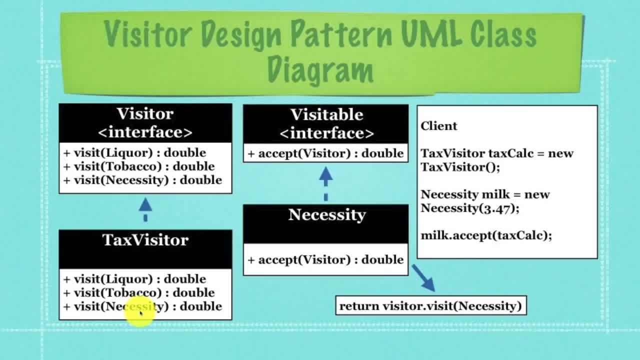 necessity. So I'm going to use this very specific form of the method: visit and I'm going to perform a tax calculation, bounce that back as a double and then that double goes right here. which we can of us to do is to create completely different ways of taxing different 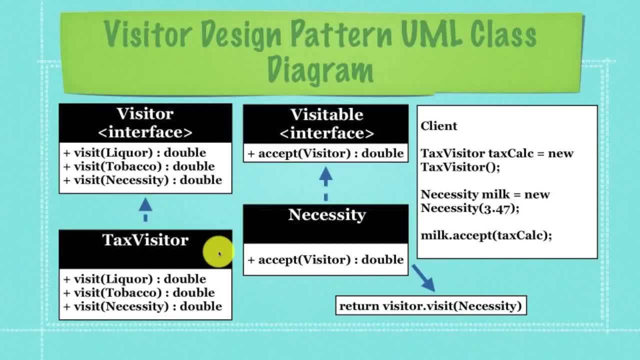 objects, as well as very easily implementing new ways of taxing just by implementing the visitor interface. So let's get into the code and show you an example of exactly how this whole thing is going to come together. So here we are. this is a visitorjava, which you saw previously, and all the code in this. 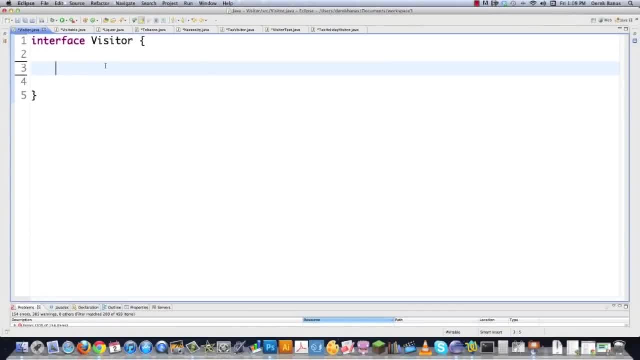 video is available underneath of the video in the description area, and you should definitely take a look at it because it is heavily commented. Now, this is going to be an interface called visitor, and it's gonna be very, very simple and it's just gonna allow us to perform the same action on many 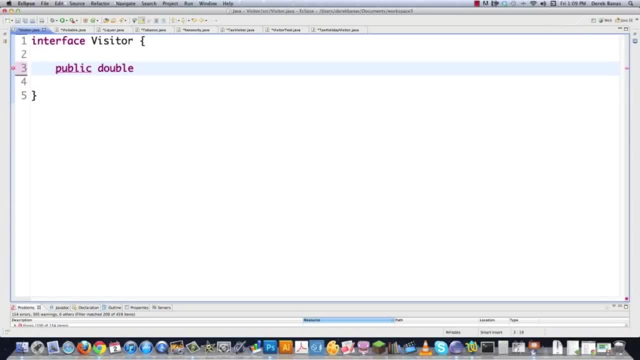 different objects of different types. So we just need to go public double visit and then here we're going to handle if a liquor object is passed over right like that, and then what we need to do is use method overloading to allow us to accept other different types of objects that are passed over. So here we'll have. 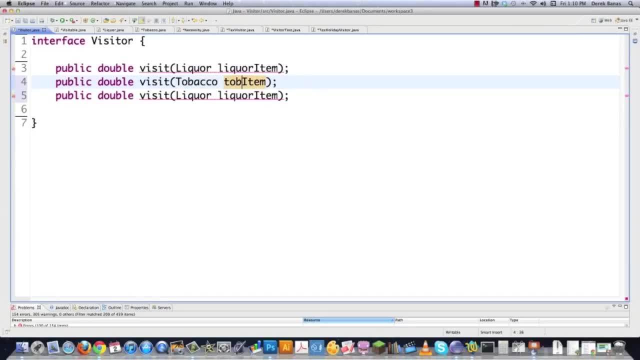 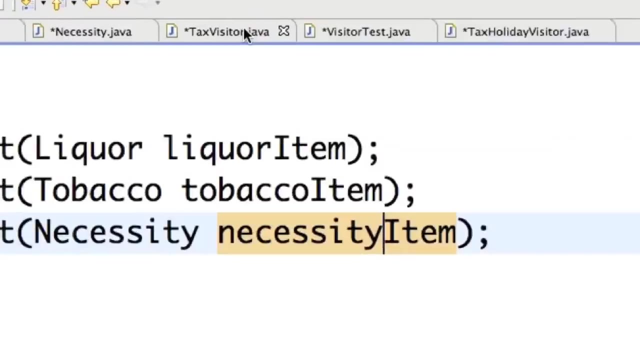 tobacco, and then let's just say this is a tobacco object, And then also we'll be able to handle necessity objects, which would be like food, and then we're gonna call this a necessity item. There you are, you done with that visitor interface. Now we're going to go into taxvisitorjava. 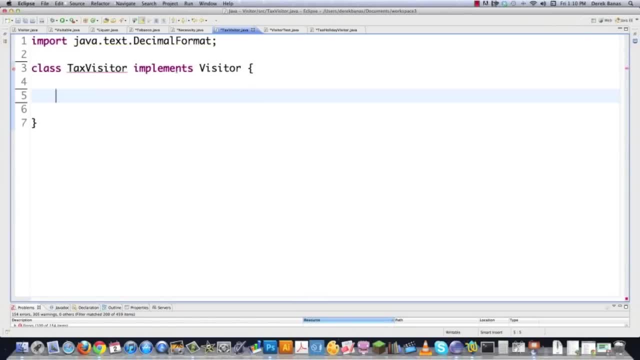 which is going to implement this interface and, as you can see, I did that right here, and up here I'm gonna be changing decimal formatting so that I can show cents in just two digits. So here's tax visitor and implements visitor which we just created previously, and let's just get the decimal format. 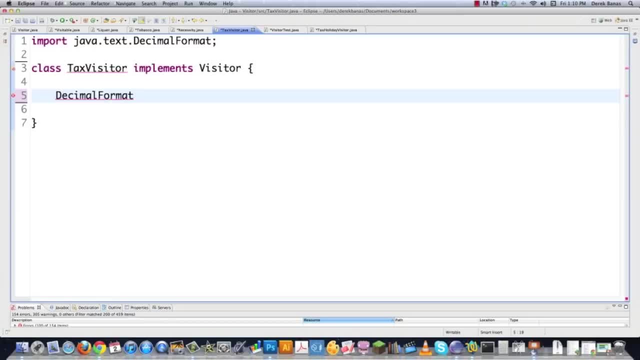 here. So here's tax visitor and implements visitor, which we just created previously, and let's just get the decimal formatting thing out of the way, because it really doesn't have anything to do with this, but I just thought it would be important to use. So there's decimal format and 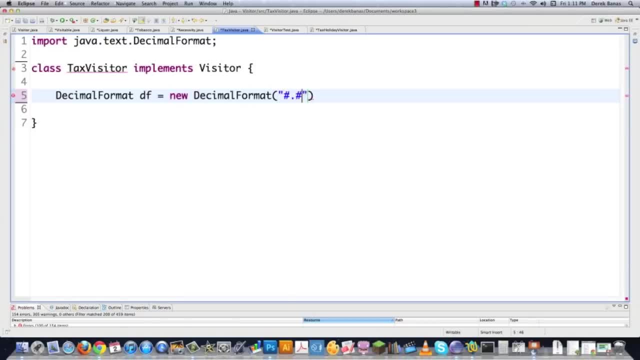 then here we're going to say that we're going to accept one or more digits and then there for our cents. Then we're going to come in here and go public tax visitor, which is the constructor for this guy and in essence he's gonna do. 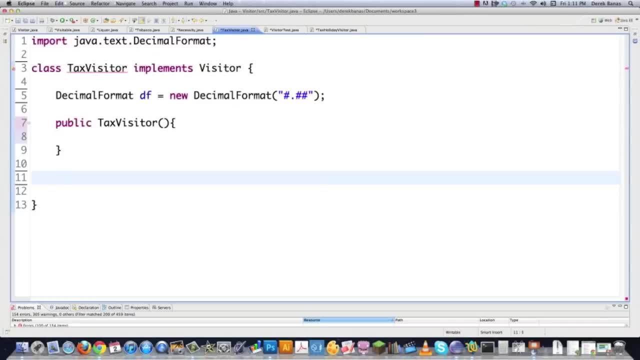 nothing, He's just going to sit there. I could do all kinds of things with him and you might decide later on you want to, but for now that's just gonna sit there. Then what I'm gonna do is go up to tax a visitor and 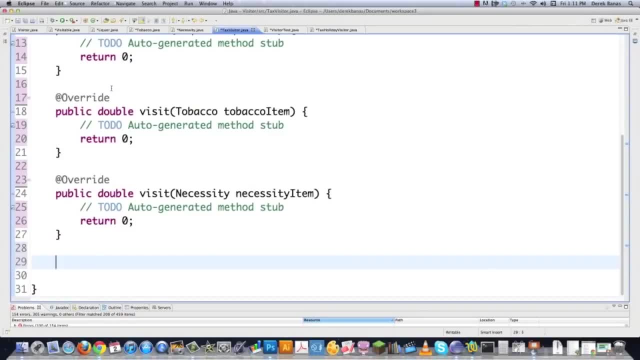 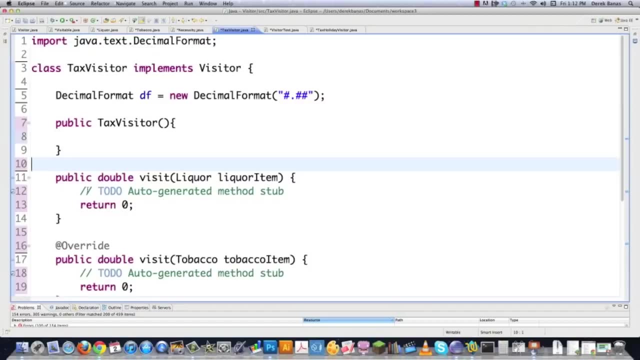 it's gonna say: hey, there's some methods you need to add in here. I'm gonna click on that and create all those, so I don't have to type it out, and then I'm just going to override these to make them do exactly what I want them to do. So in 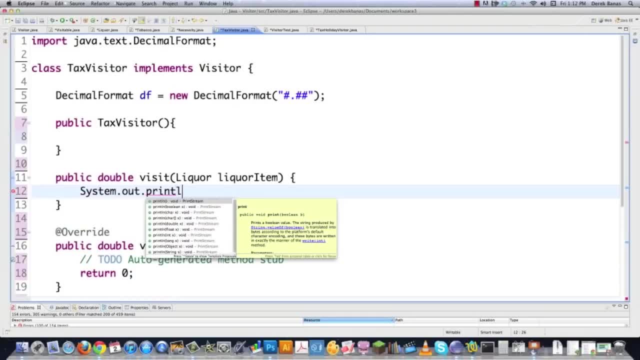 this situation. I'm gonna go system out print line and say this is a liquor item price with tax is gonna be shut out. and then I'm gonna go return and then I'm gonna do a couple things here. I'm gonna say double, parse int, parse, double and 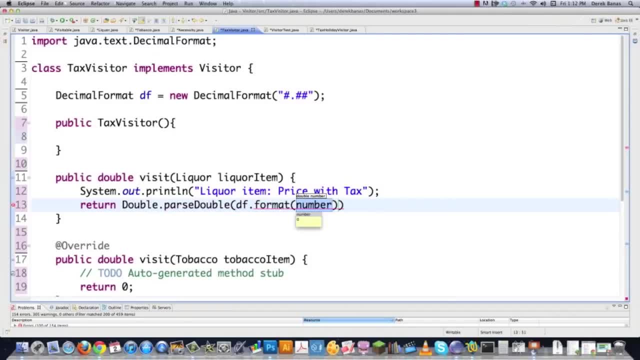 then do DF format. The reason why I have to convert this into a double is because DF format shoots out a string and then for just liquor items, I'm going to get my price and multiply that times 0.18, which is going to be the. 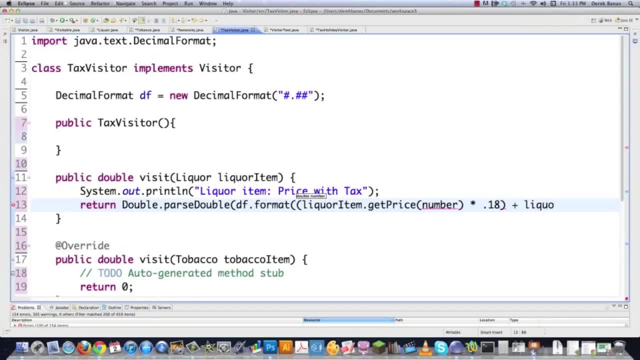 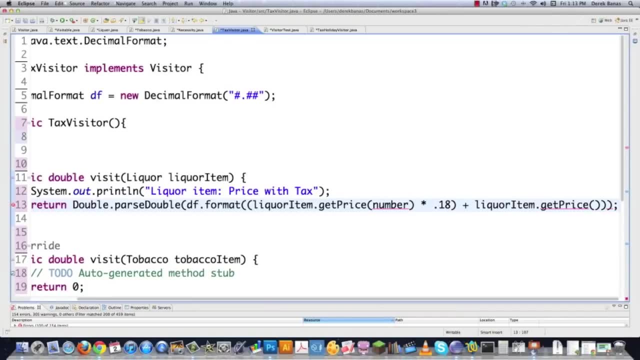 taxation on liquor items. and then I'm gonna go liquor items again and this just provides an easy way for us to be able to calculate tax in a completely different way without altering the classes themselves. So that's why that guy's there and then get price. doesn't need to have anything inside of it, Okay. 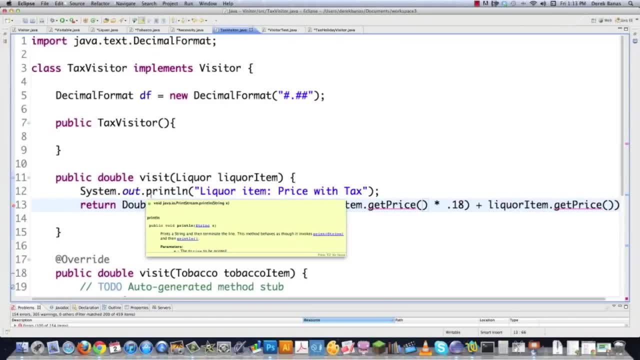 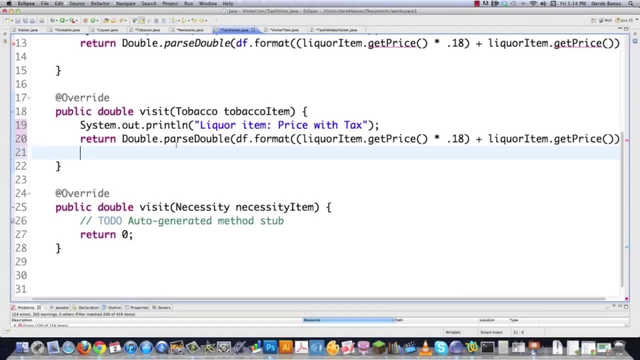 so you can see exactly how visit is gonna work in here In this situation. and guess what this? it's gonna work in almost exactly the same situation if a tobacco item is shot over here, So we're just gonna paste that inside here and all I need to do is go tobacco item price with tax and then. 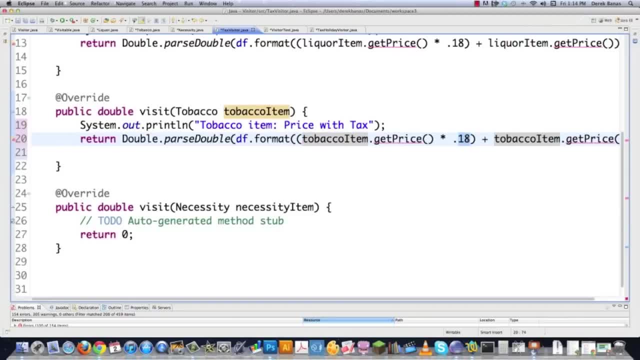 this is gonna change to tobacco item, and then we're gonna change the tax on that- just that specific item- to 32, and then we're gonna do exactly the same thing for necessity items like that and like that, except in this situation we're gonna say that the necessity item doesn't have any tax, just to make it. 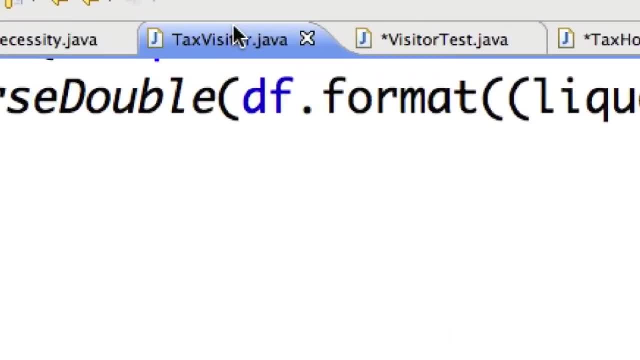 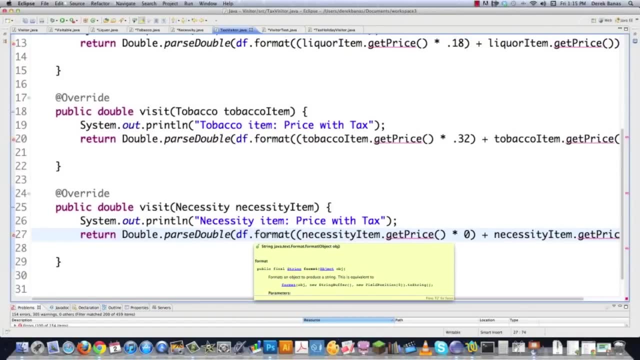 simple and show something completely different. So there you go. there's tax visitor dot Java. so now what I need to do is go in and actually show you what these classes would look like before they were ever created and the changes that are gonna be needed to make them work. So what I'm? 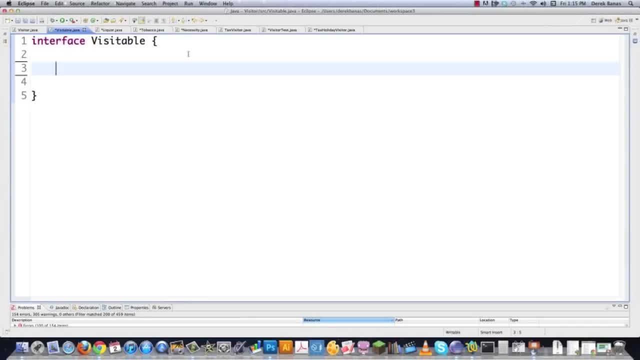 gonna have to do here is create what's called visible dot Java, and this is another interface, and inside of this, very simply, I'm just going to go public double, and this is the only change it's gonna have to be made to your classes to be able to implement the visitor design pattern. So now let's go into a liquor. 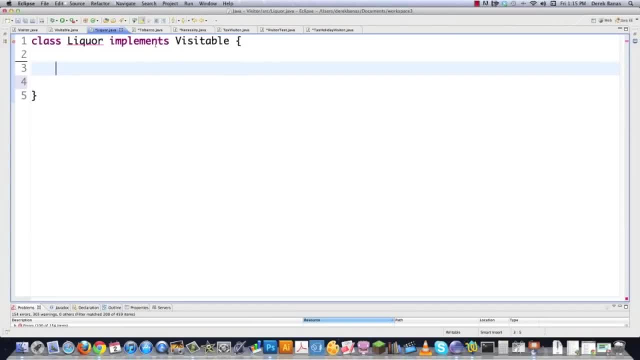 dot Java and show you exactly what it would look like before visible was ever even created. So let's say we have private double price and the way that this used to work is taxes didn't exist. so we're just gonna say: okay, we're gonna get a double passed over to this like that, and then we're just gonna say price. 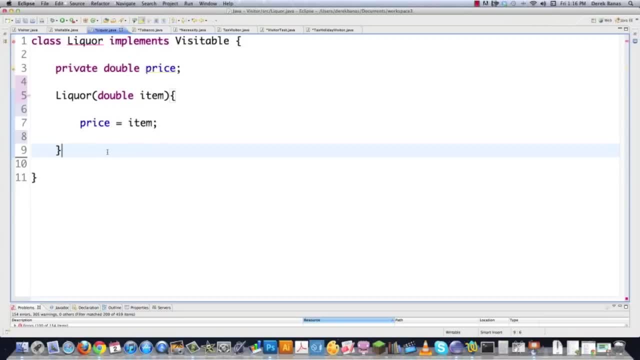 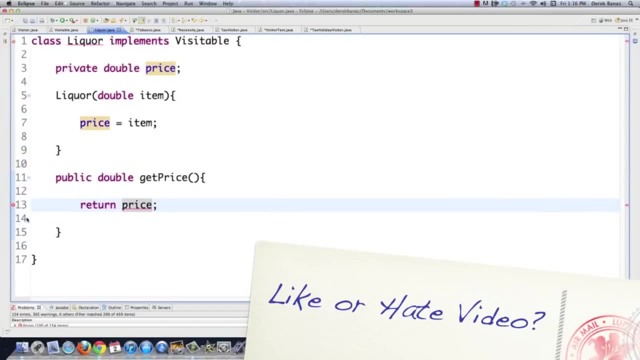 is equal to the item price that was passed over. and then we're gonna say: public double get price, return price. Okay, so this is the way that all of these methods were created. So let's go back here and let's go back to our different classes, and then we're going to look before: visible was every ever. 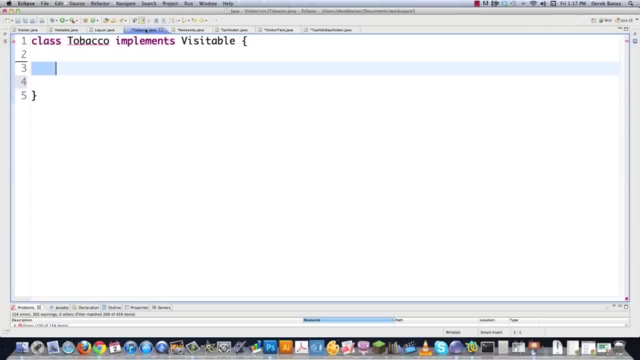 implemented. So let's actually go and create all those. So let's just go copy. let's jump into tobacco. do pretty much exactly the same thing there, that is, except this, of course, needs to be tobacco. everything else can stay exactly the same, and then we'll go into necessity items, and that also is going. 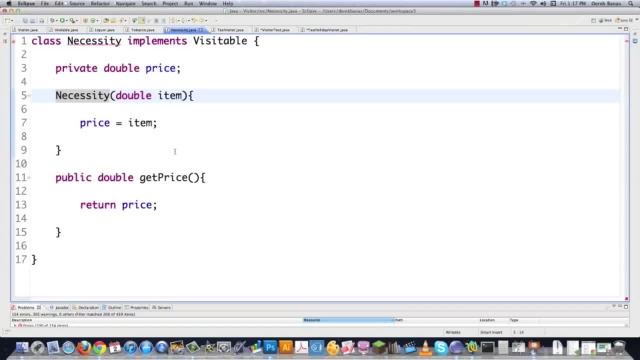 to be exactly the same And that all works. now, what happens in the situation where now, all of a sudden, we have to implement taxes? Well, we could come in here to each one of these classes and create that capability right here and had capability for calculating taxes. However, the problem is what happens whenever we have to? 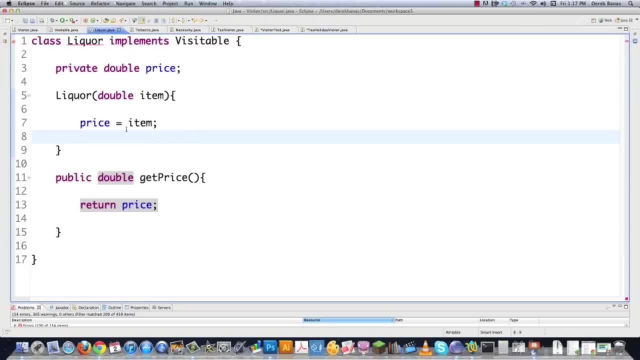 implement even more different capabilities to these classes. We're going to have to keep going into every single one and changing them over and over and over again. Or what we can do is use the visitable interface that we just implemented here in this guy And we just come up here and say add: 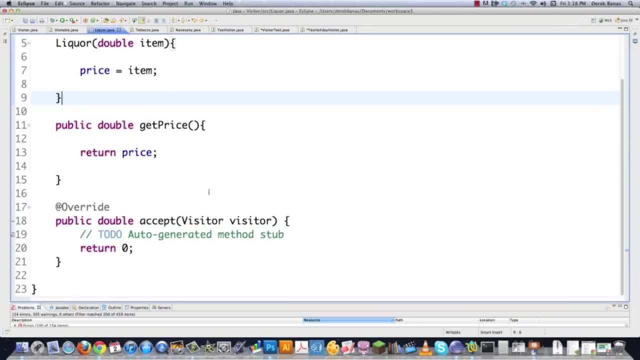 unimplemented methods. And then we hit file save And now what we can just come in here and do is go return visitor dot visit and then pass it over to this, which is a reference in this situation to this class, which is liquor. So that's going to be passed over to this guy And this can be used over. 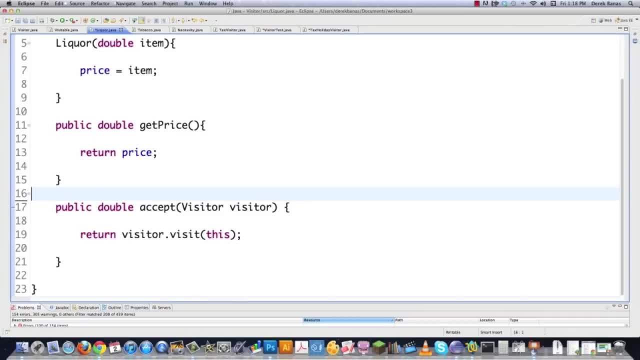 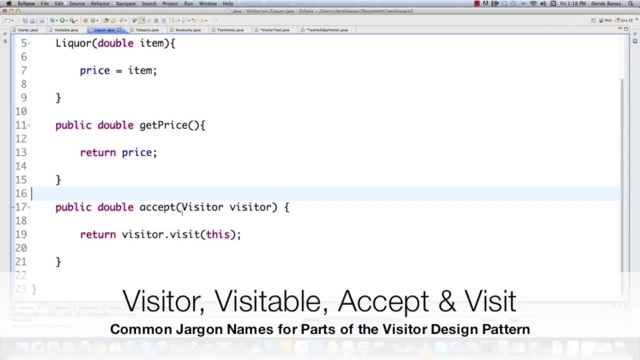 and over and over in multiple different ways and execute multiple different methods, And this, of course, doesn't need to be called except I'm using that because that's a common jargon way of referring to these guys. But you can see, here, if I pass over this meaning liquor, then it's going to. 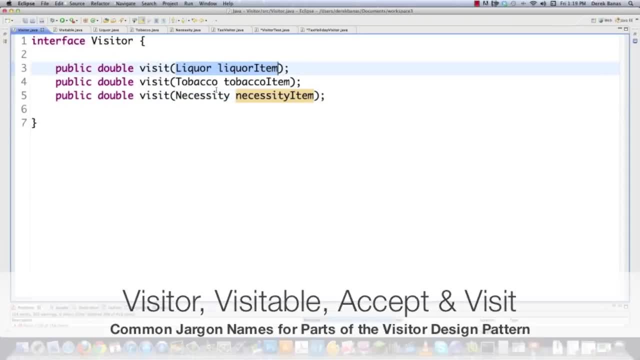 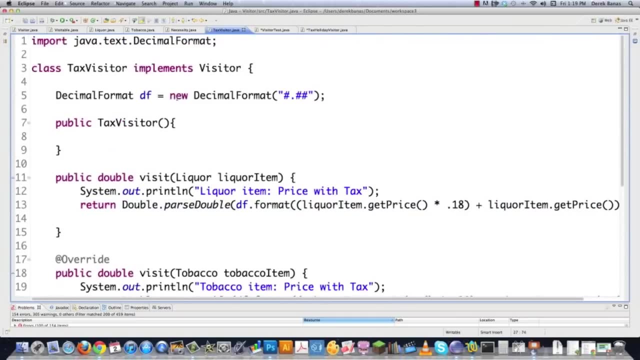 jump over into this guy and it's going to say, okay, this is a liquor And we need to perform certain calculations based off of that fact. And then it's going to go down here to tax visitor, which implements the visitor interface, And it's going to come down here to 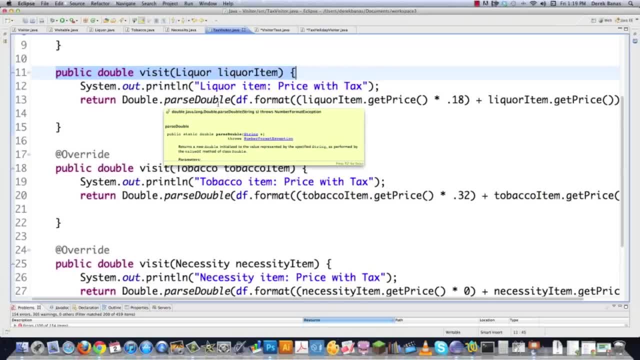 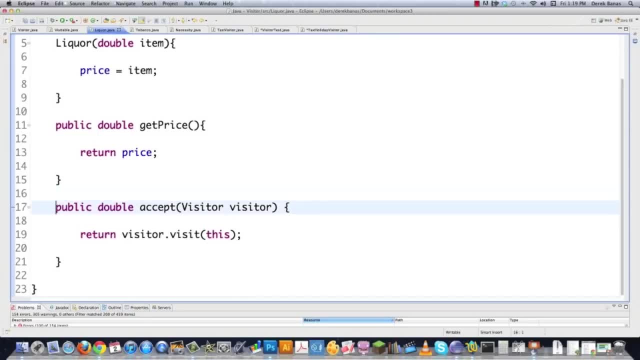 liquor item and perform this very, very specific calculation just for that type of object. So that's what's going on with that And you can see here it's very, very simple And accept is exactly the same in every single one of these objects. So let's copy it and we can come in here and paste. 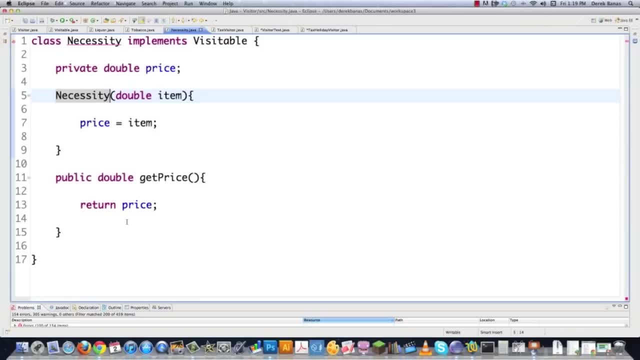 that in. Okay, now that works, And then we can do the same thing for the other object, And we can do the same thing for the other object, And we can do the same thing for necessities, And we don't have to care at all about anything, Just let the accept method handle. 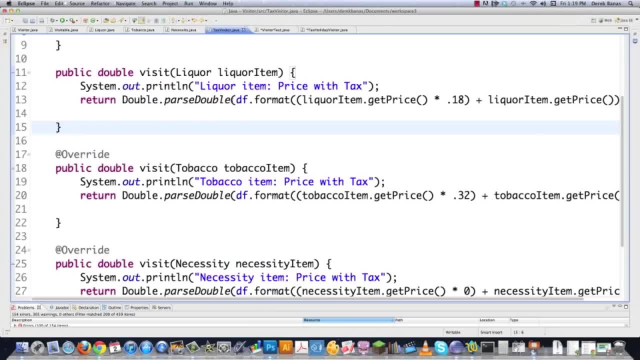 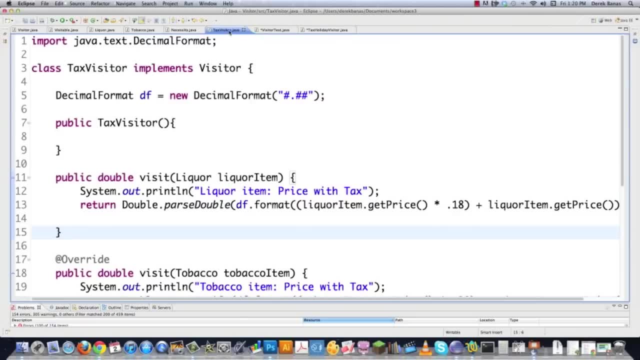 everything for us. And then what's cooler even yet is we could have multiple different types of calculations. So let's say that the government wants to institute some type of tax holiday provision. Well, we could handle that. So let's just go into tax visitor and show you exactly how. 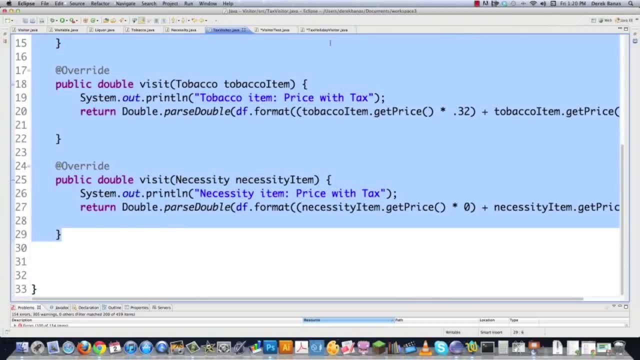 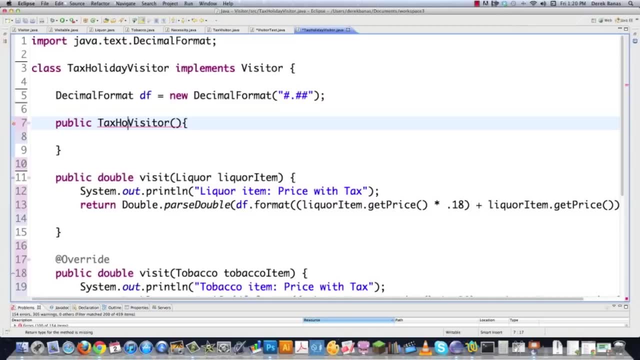 easy it would be to do that. We're just going to copy what's already been done right here, Jump over into tax visitor, Paste that inside of there And then this is all the same. However, this is going to be tax holiday visitor. Don't need to change anything else. I mean, everything else is. 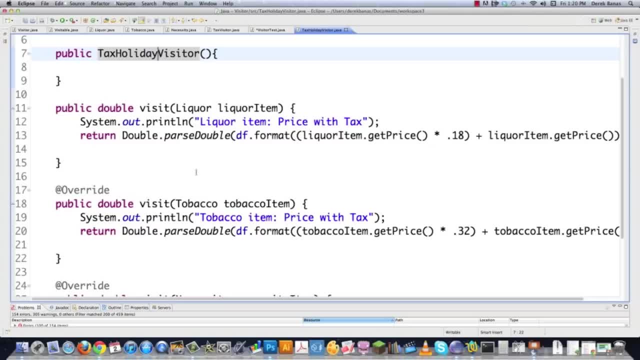 exactly the same. And then we can really really quickly come in here and say, okay, let's drop the tax on liquor to 10 during our tax holiday And tobacco to 30. And then necessity items don't need to change because they're already at zero, And then we can file: save those. Now we just 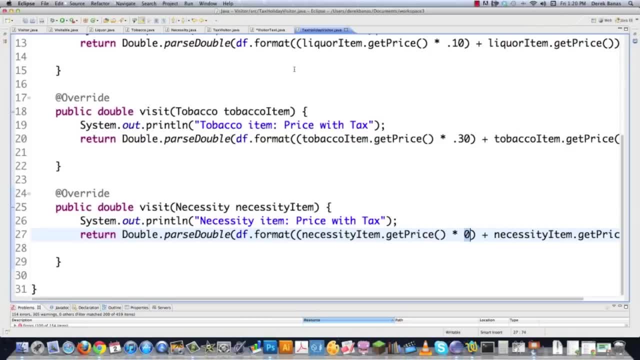 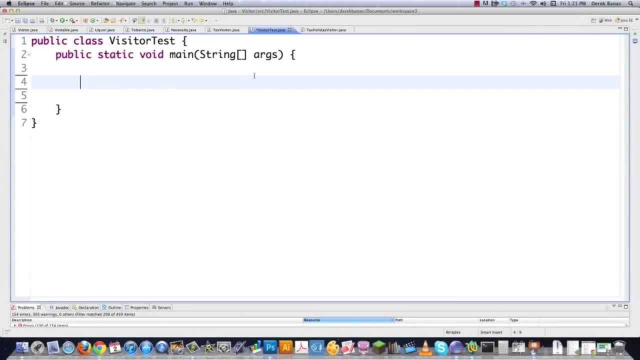 implement it in a couple clicks, A completely different way of calculating taxes And, as you can see, overall this whole thing came together quite quick And then we can go into visitor, test dot java and actually see what we got right here. So we'll go tax visitor And I'm just going to call 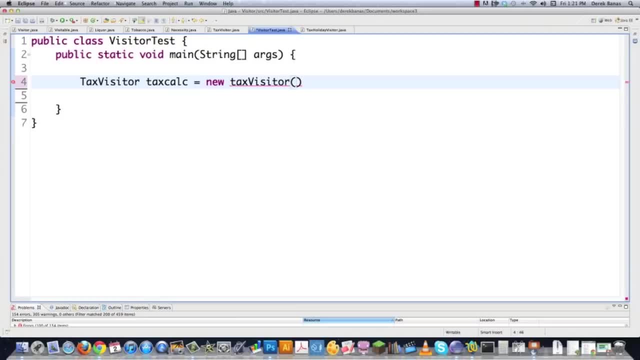 this tax calc is equal to new tax visitor. This is all about speed. That's the whole reason why you're going to use this guy And also not be having to change anything in regards to your classes, And then we're going to have tax holiday visitor And we can perform completely different. 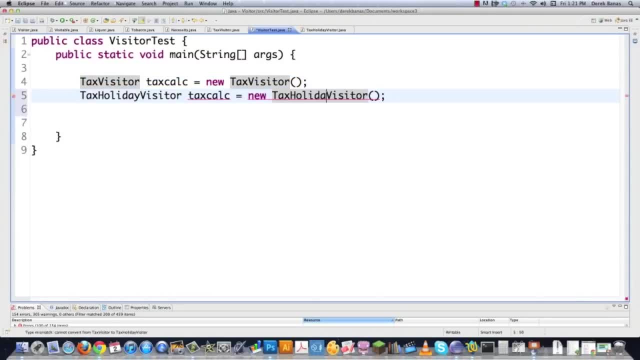 calculations in that situation. Just type in holiday there, Holiday there, And then change that And you can see really quickly how we're able to do all this. And then we're going to be able to go necessity and say milk, for example, is equal to new necessity And say the price on it's. 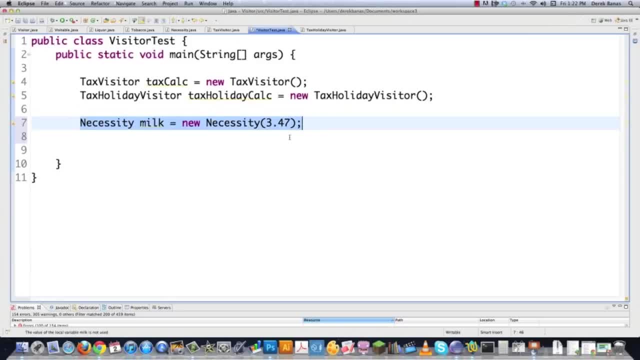 $3.47.. Right, like this, Pretty simple. And then we're going to do the same thing for liquor, And let's just say vodka- And I have no idea how much vodka costs- Let's just say $11.99.. And then 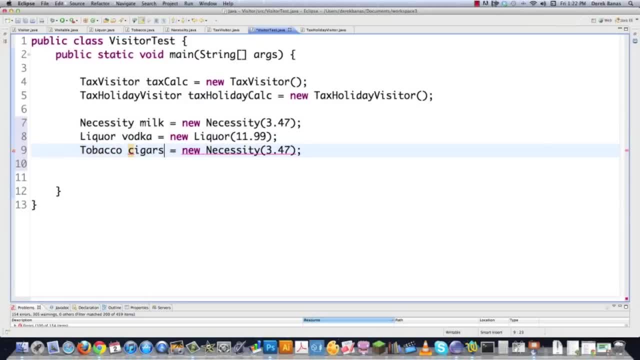 tobacco, And we'll just say cigars. And I also don't know how much cigars cost, So let's just say box of cigars, I don't know. So there you go. We created our different objects And now, if we want to be able to print out our changes in taxes, It's going to be very, very easy. We're just going to. 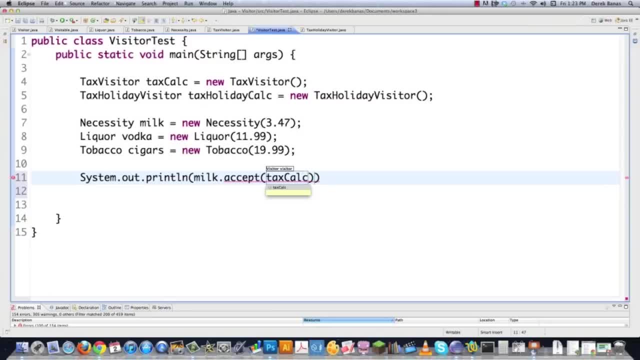 say, milk Accept And pass it tax calc, Which is going to be our calculation we want to use at this point in time, And then, just to keep everything spread out, I'm going to throw a new line inside of there And then I'm going to be able to copy that And then just change this to vodka And 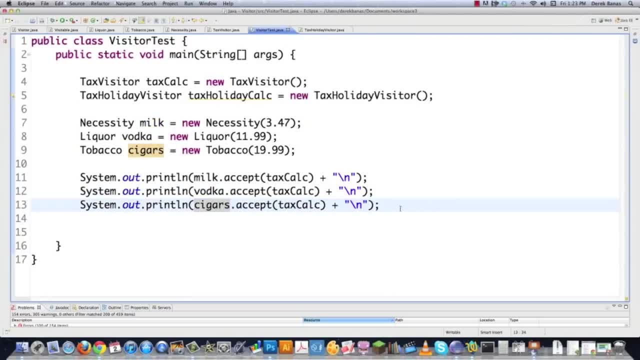 then change this to cigars. Didn't have to change anything else, So that's pretty cool. And then we could also come in here and do something else, And then we're going to be able to print out our changes. So we're going to do something like tax, holiday prices, And then we're just going to 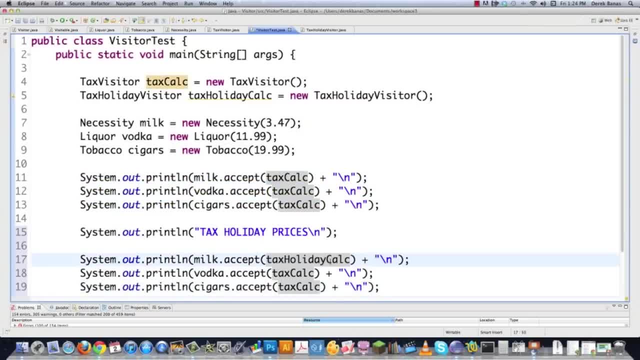 copy these three guys right here, Boom. And then we can come in and say: holiday, Tax holiday. And then we can copy that, Paste that in there And paste that in there. So you just created two completely different ways of taxing actually Six. And then if we execute this guy, you can see: exactly how it's going to work And that's exactly what you see. See necessity items. Price with tax: $3.47.. Liquor price: $14.15.. Da, da, da, da da. Of course, necessity prices don't change. This is. 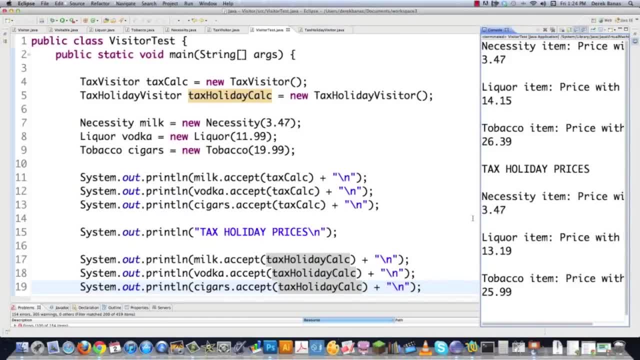 a very simple way to do tax holiday And so forth and so on. There is an extremely useful design pattern. Calls it a visitor design pattern. If you didn't quite get it, take a look at the code- Really meticulously look at it, And I guarantee you're going to get it. So what comes up next? 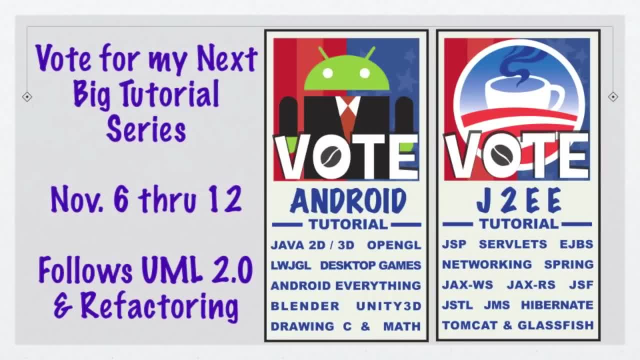 Next week, for the people that watch my videos all the time- All 150 of you guys- I'm going to hold a big, giant vote. I basically have two groups of people out there who want two completely different types of tutorials, Both of which are completely huge. So, from November, the 6th- 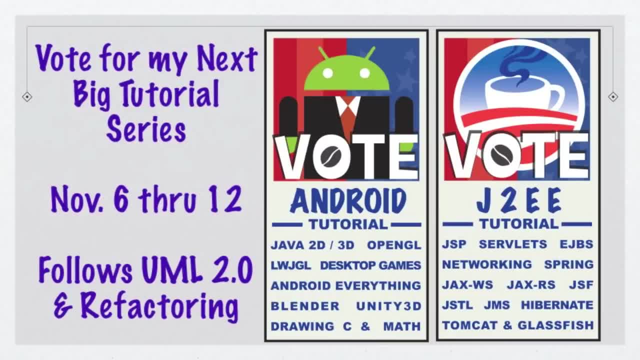 Through the 12th of next week. I'm going to allow you to decide, Based off of just a simple vote, Which one I'm going to cover. I'm either going to go down the Android game path, Which is also going to include the C programming language, drawing A whole bunch of math And a whole 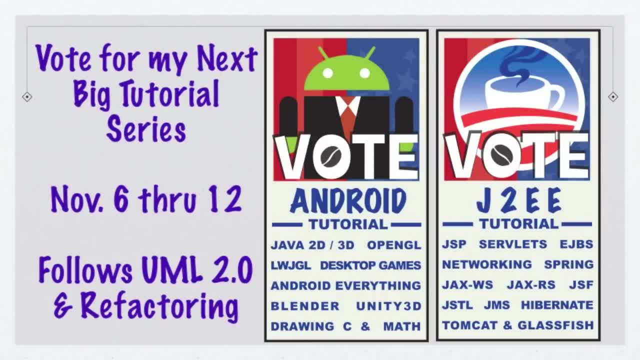 bunch of other stuff you see right there on the screen, Or I'm going to go down the Java Enterprise Edition path, Which is going to have all the things you see on the right side of the screen With a bunch of other things you don't see. that will make sense, So I leave it completely to you. 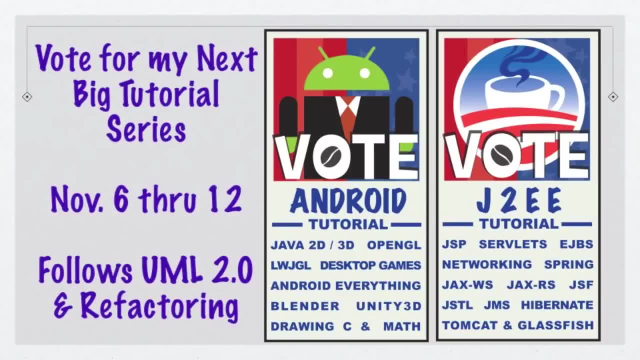 the 12th, Go out there and vote. Last time I had a vote like this That defined what I did. I had about 43 people vote, So your vote will count. And then this tutorial is going to last anywhere between six to eight months- Both of them- So you know they're going to be big, giant, massive. 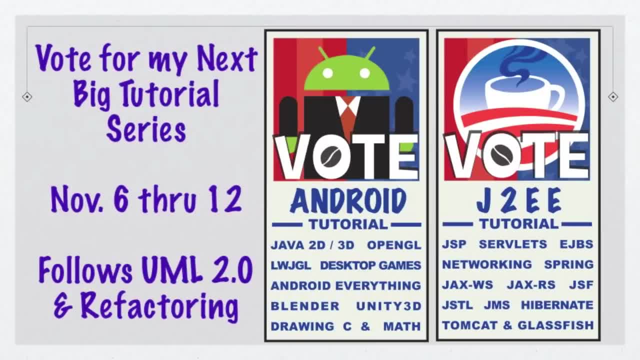 tutorials, And they're both going to start immediately after: my UML 2.0 tutorial, Which is going to start pretty much in the next couple days, And my refactoring tutorial, Which is going to answer the big question of when do I use design patterns. So there is everything.